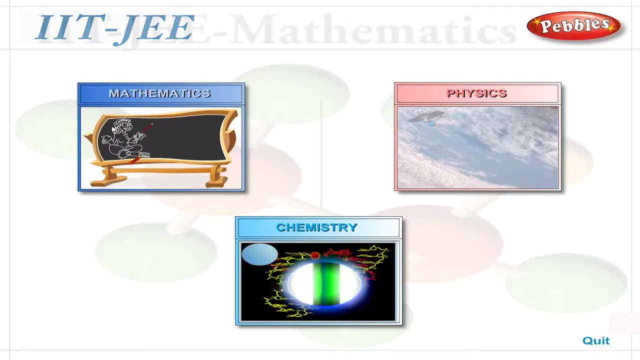 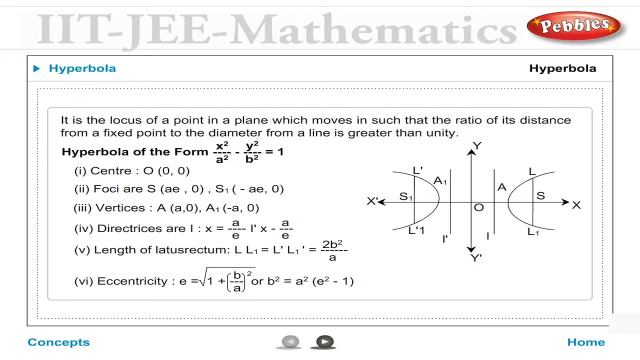 Hyperbola. It is the locus of a point in a plane which moves in such that the ratio of its distance from a fixed point to the diameter from a line is greater than unity. Another form of hyperbola: conjugate hyperbola. 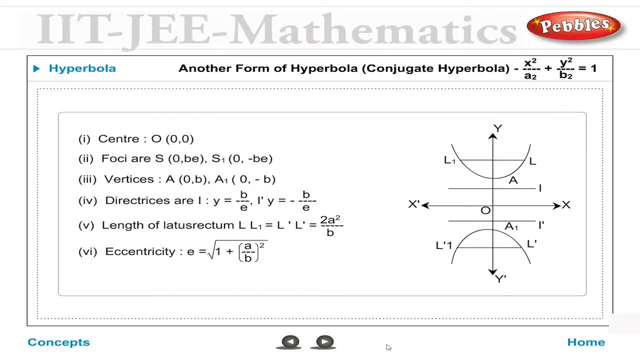 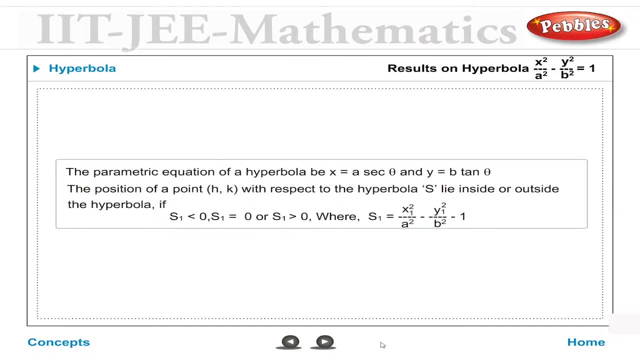 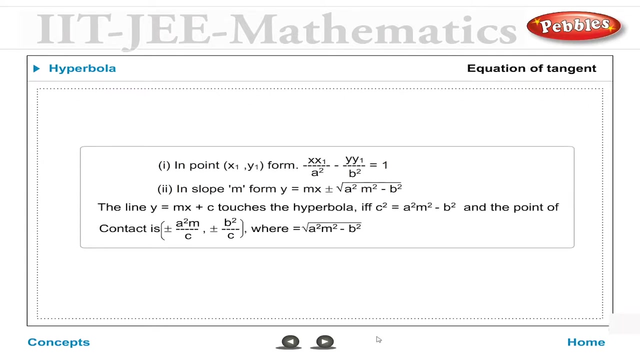 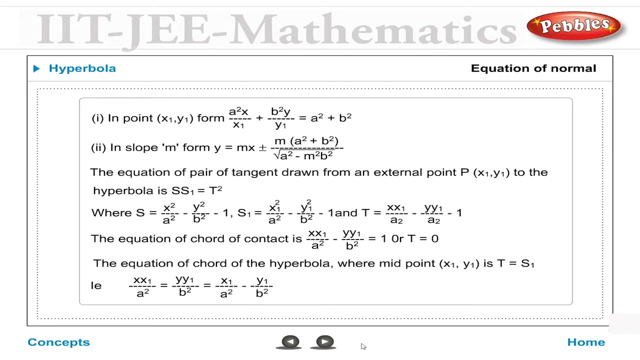 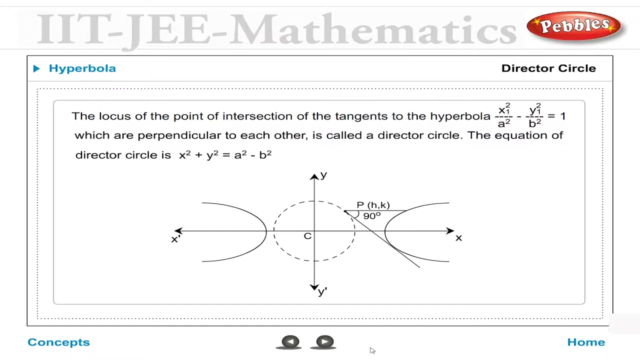 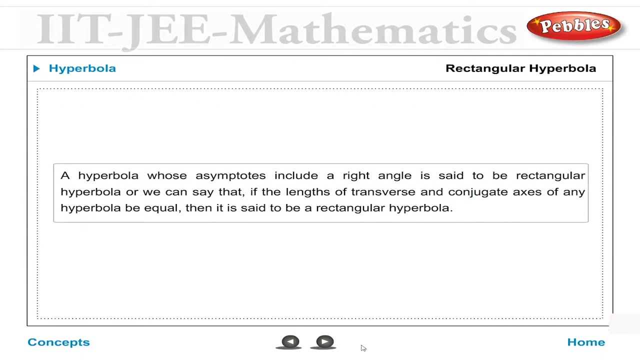 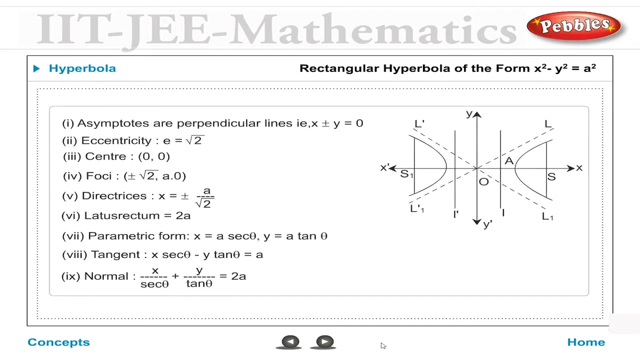 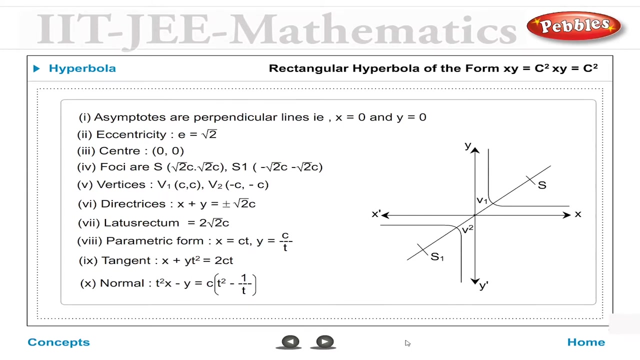 Results on hyperbola. Equation of tangent. Equation of normal Director's circle. Rectangular hyperbola. Rectangular hyperbola of the form x square minus y square is equal to a square. Regular Rectangular hyperbola of the form xy is equal to c square. 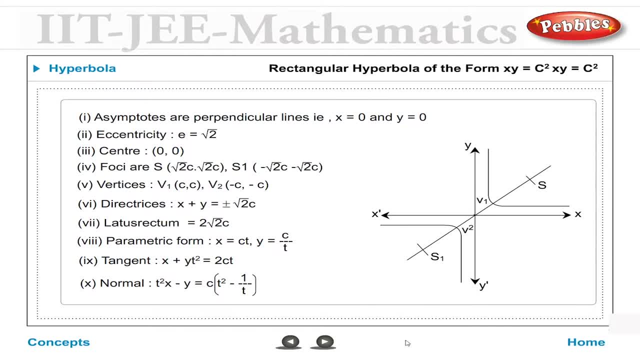 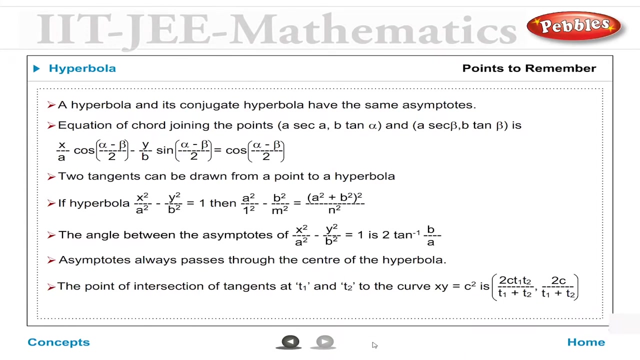 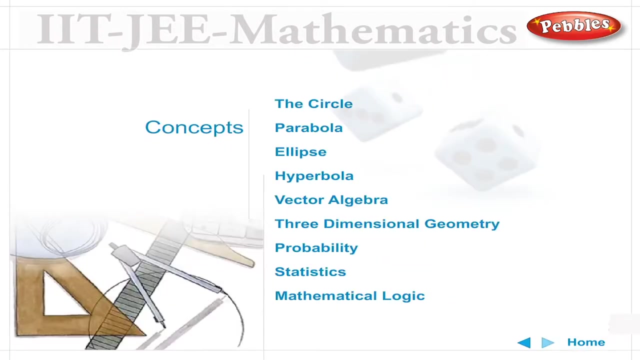 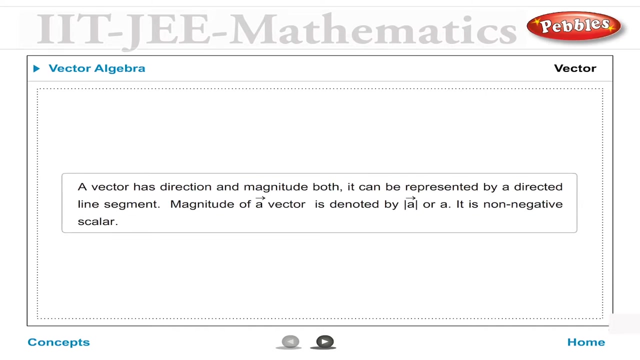 amel Points to remember Vector Algebra Vector. A vector has direction and magnitude, both It can be represented by a directed line segment. Magnitude of a vector. A vector is denoted by determinant of A vector or A. It is a non-negative scalar. 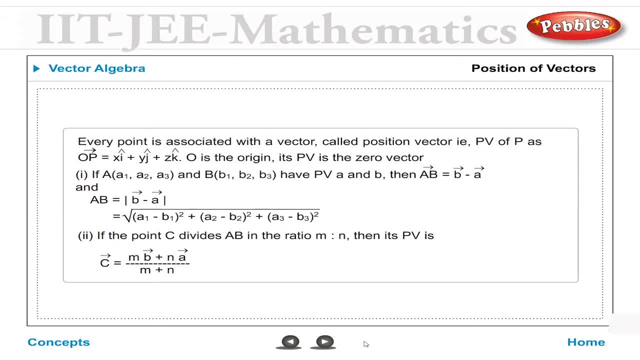 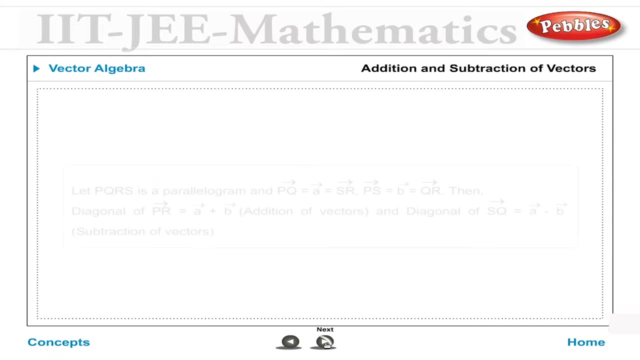 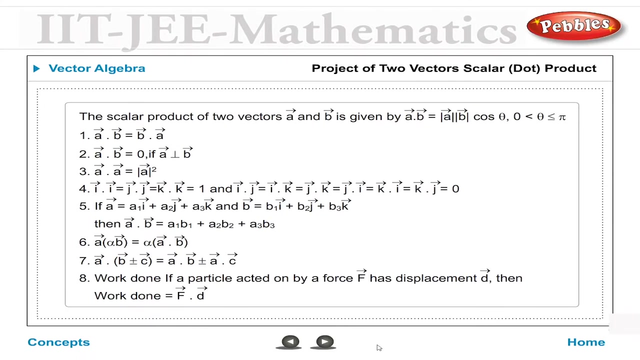 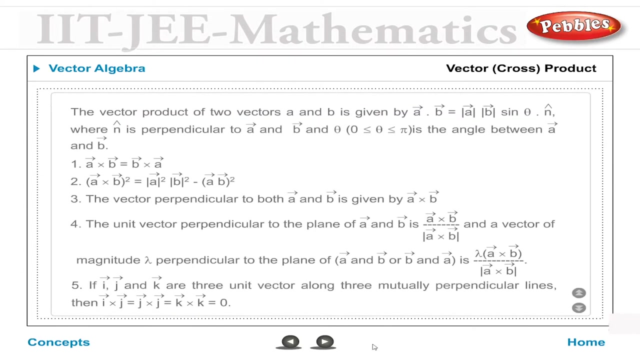 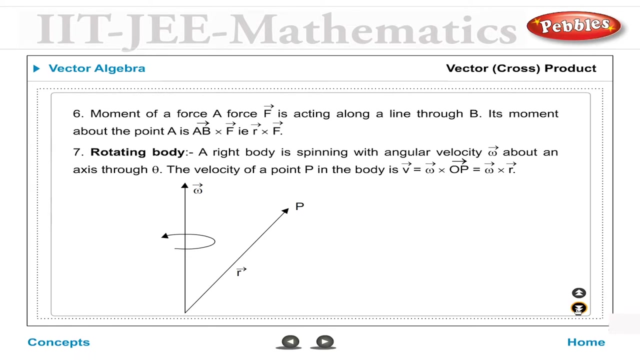 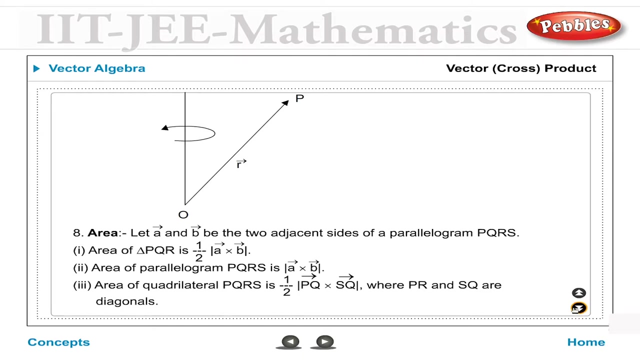 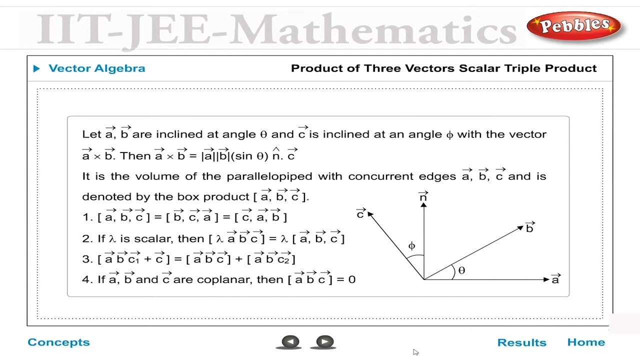 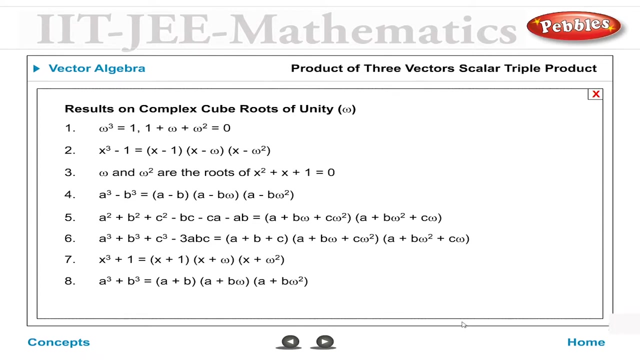 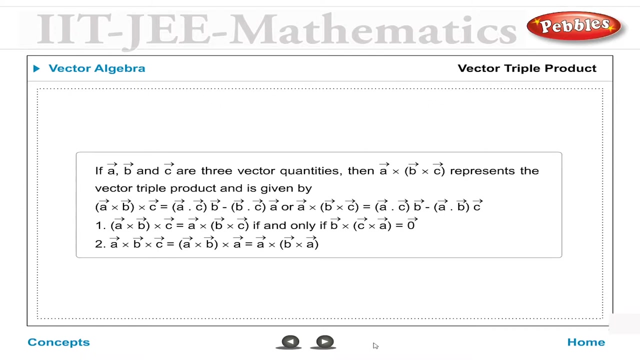 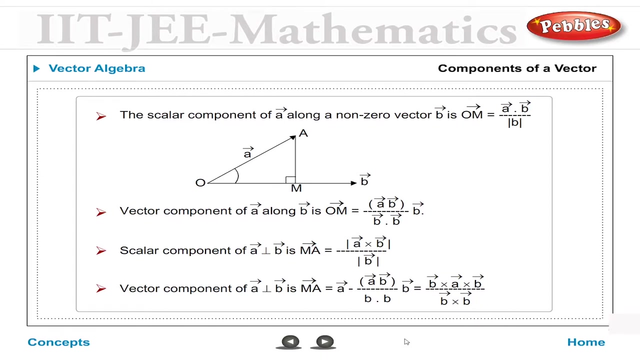 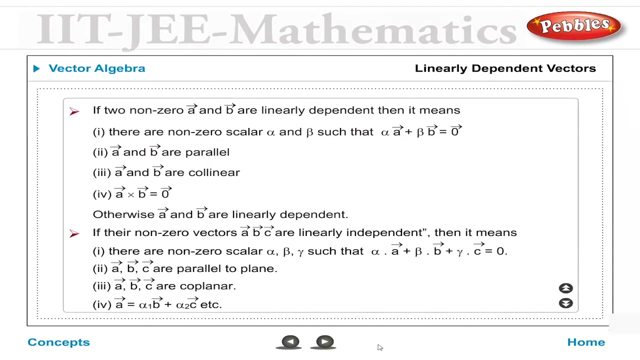 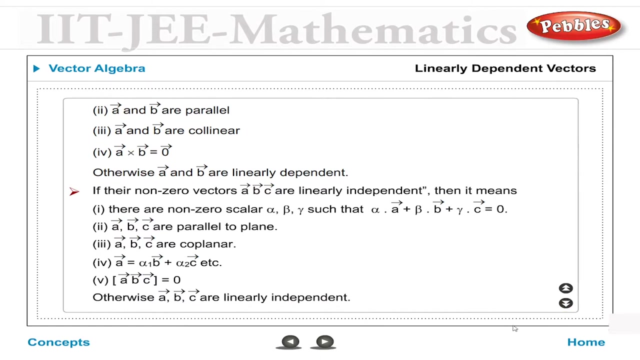 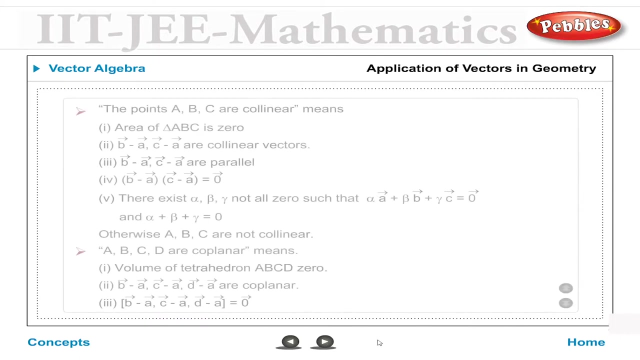 Position of Vectors. Vector double: addition and subtraction of Vectors. Project of two Vector: Scalar dot Product T. Vector Cross Product. Vector Cross Product. Product of three vectors: scalar triple product. Vector Cross Product. Vector Triple Product. Compounds of a vector. Linearly Dependent Vectors. Linearly Dependent Vectors. 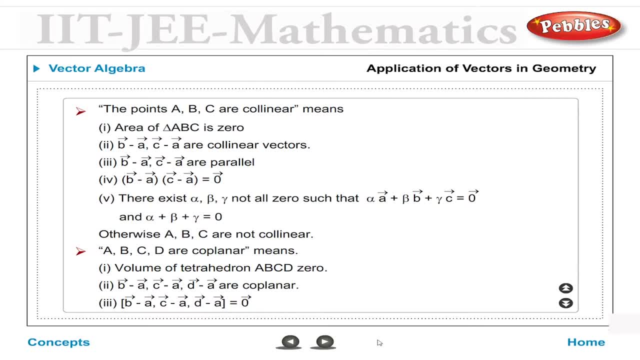 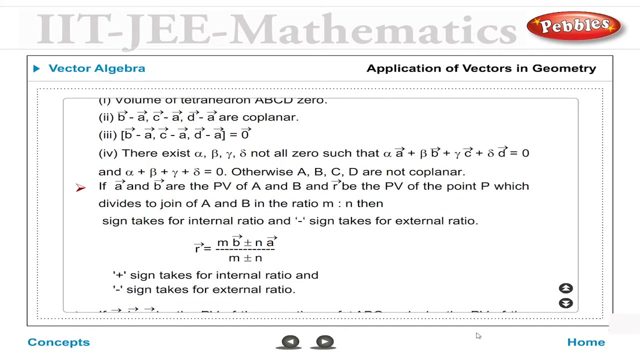 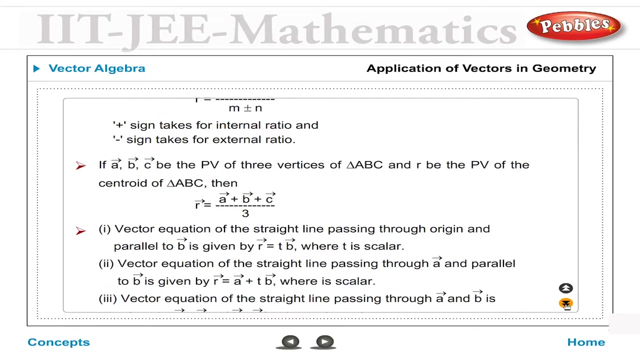 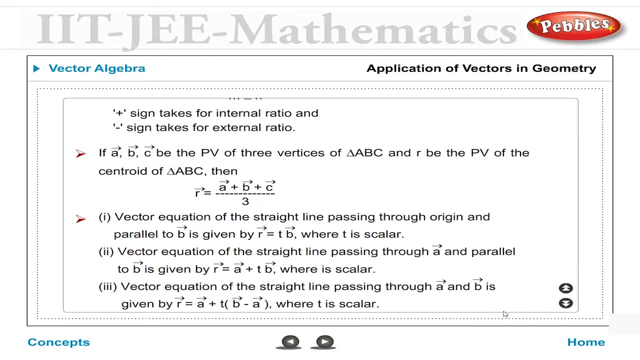 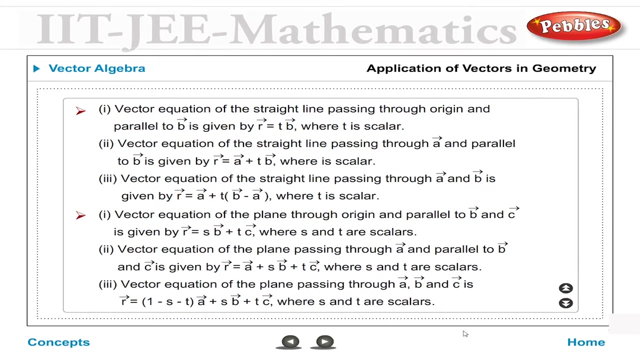 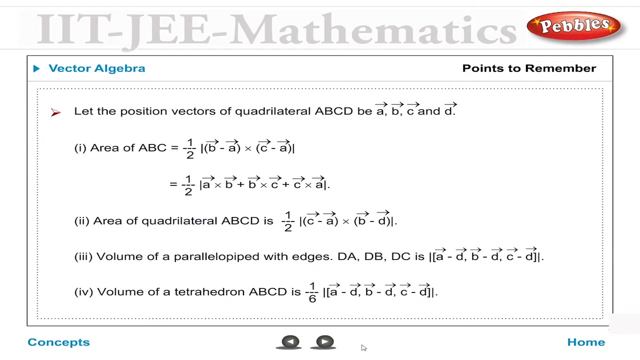 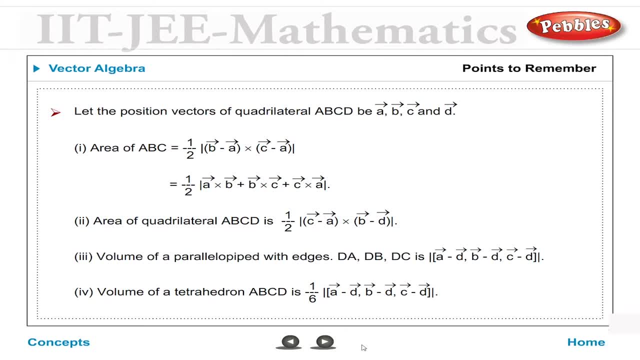 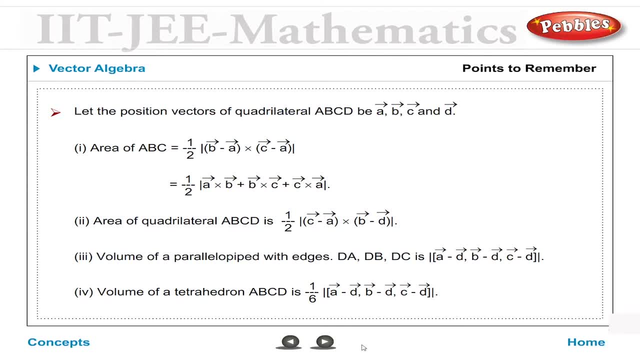 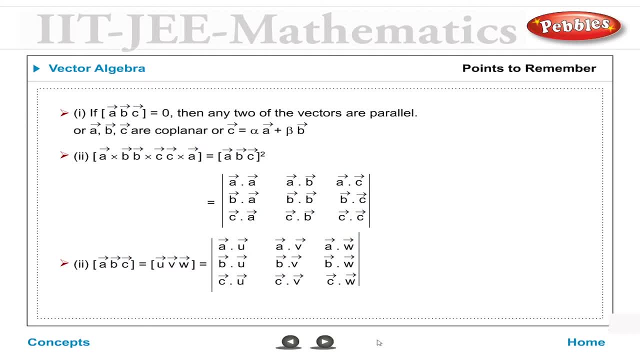 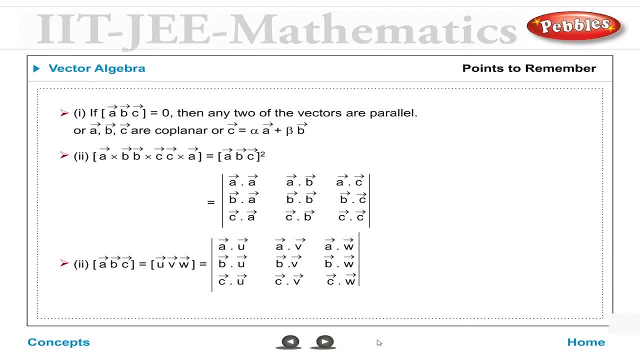 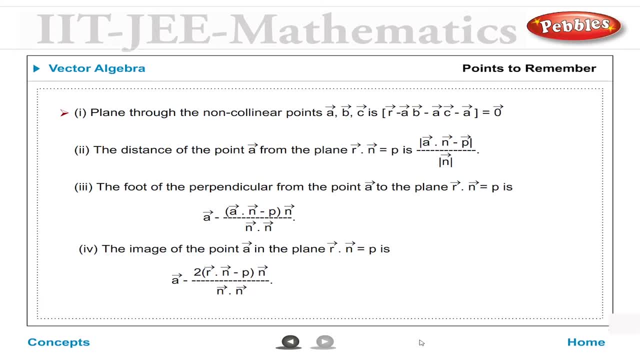 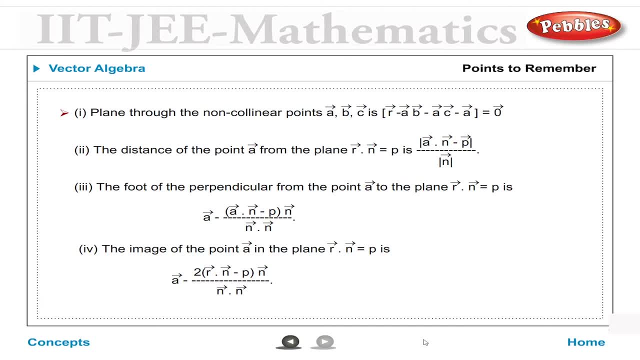 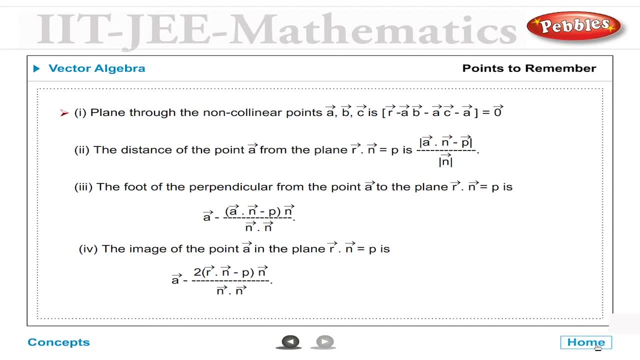 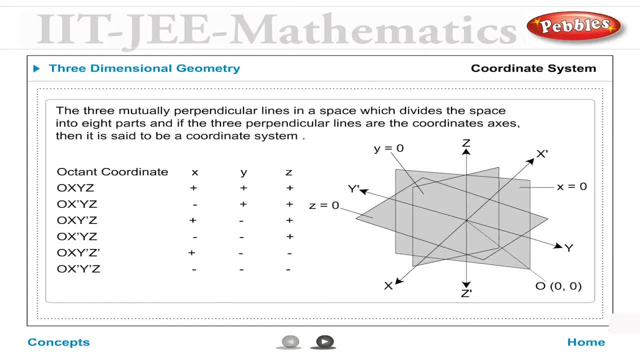 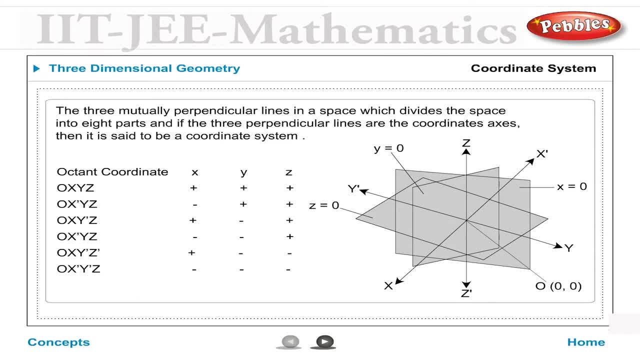 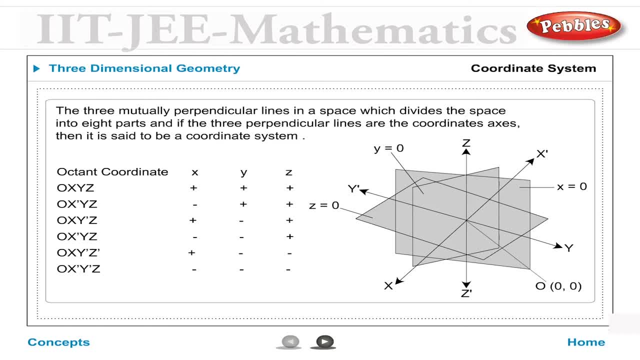 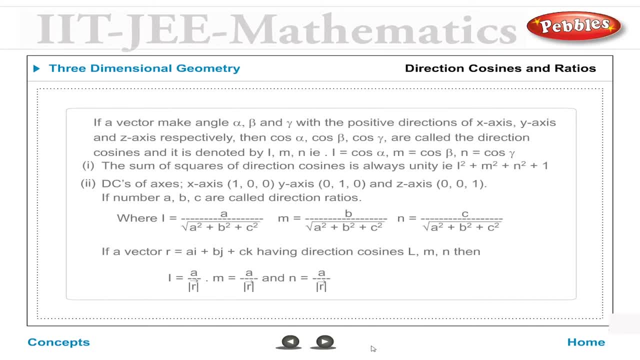 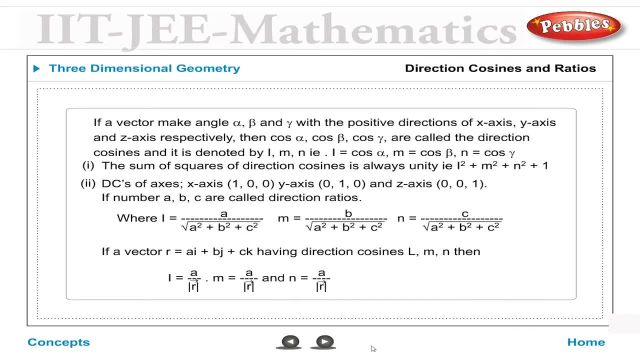 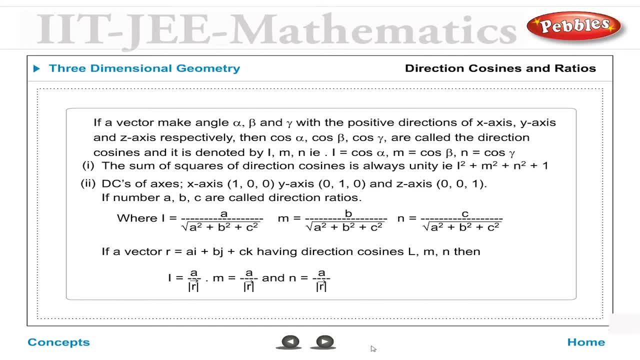 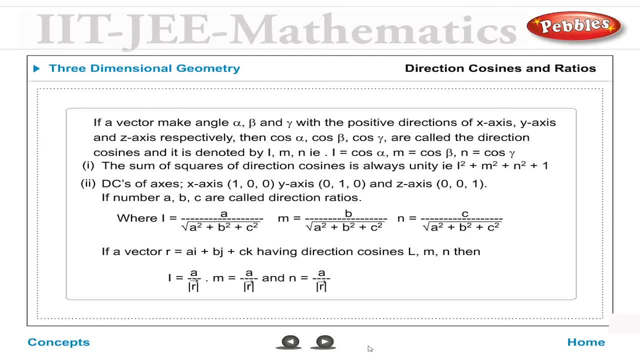 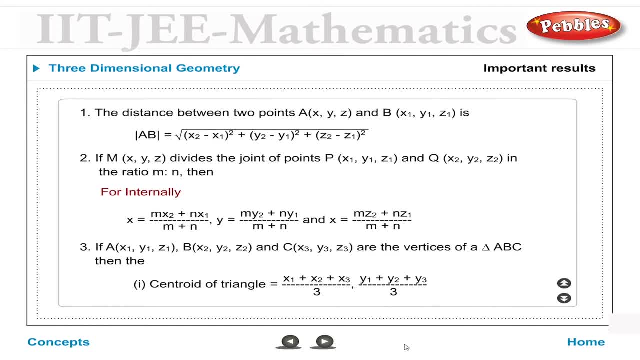 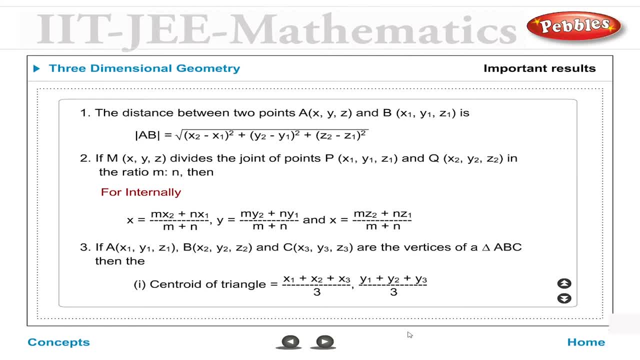 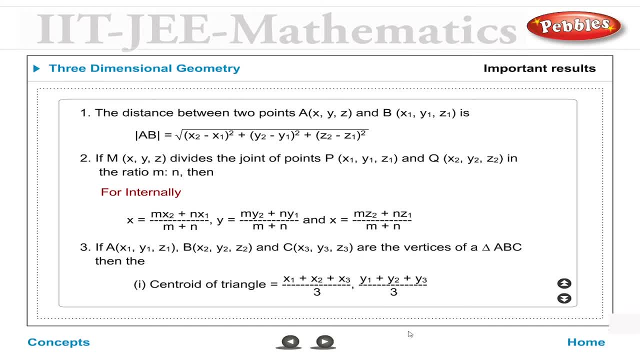 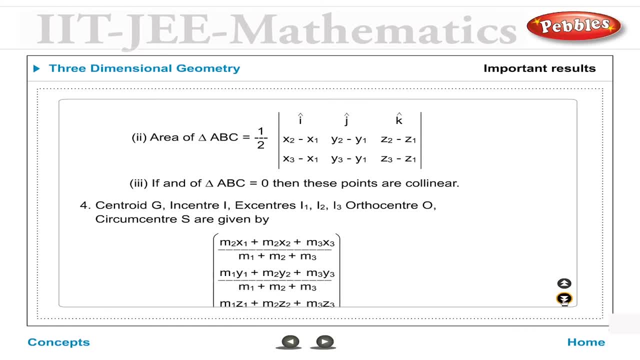 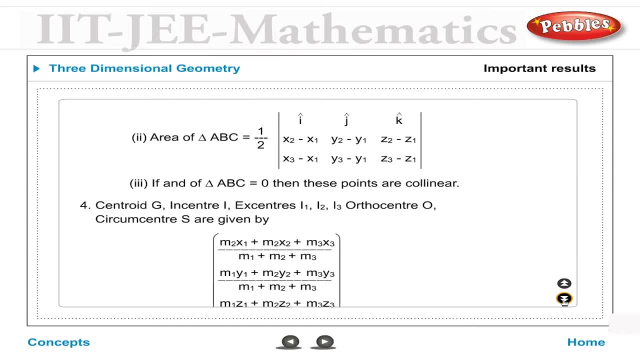 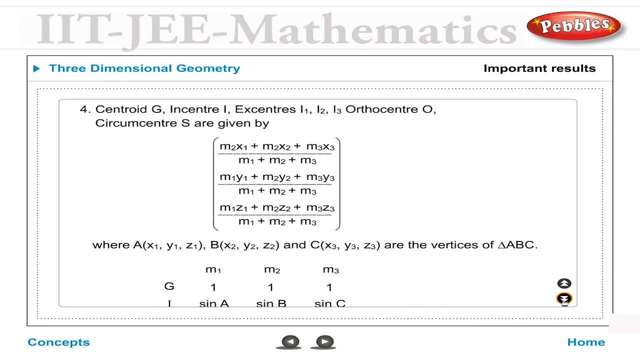 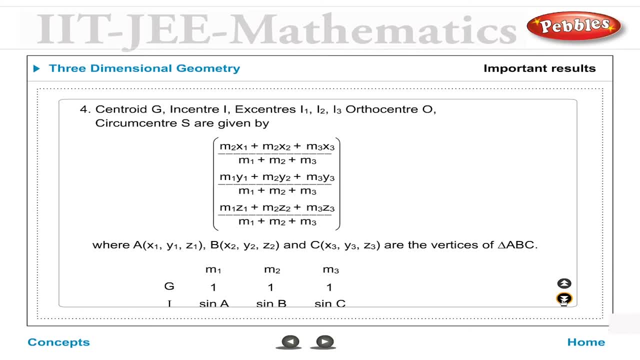 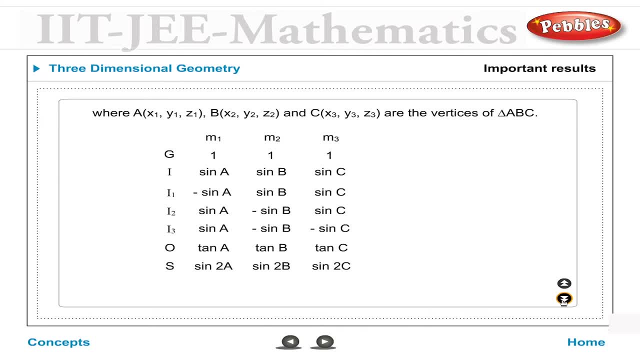 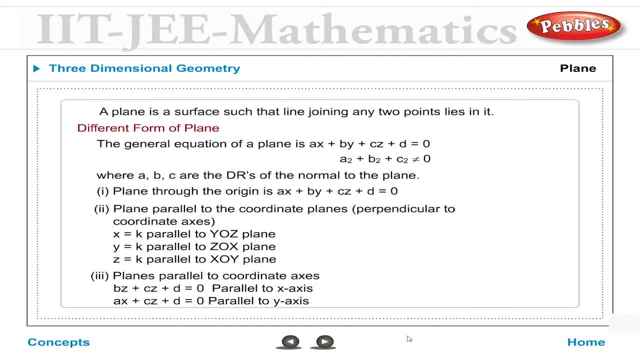 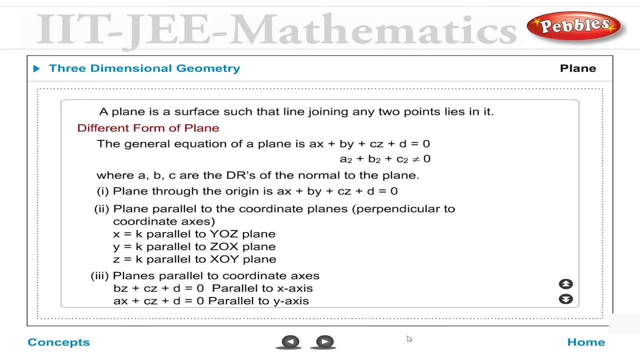 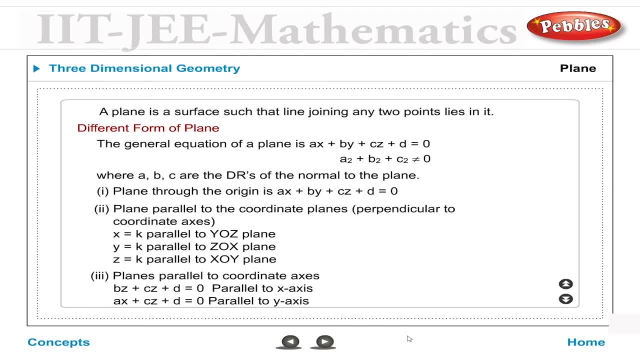 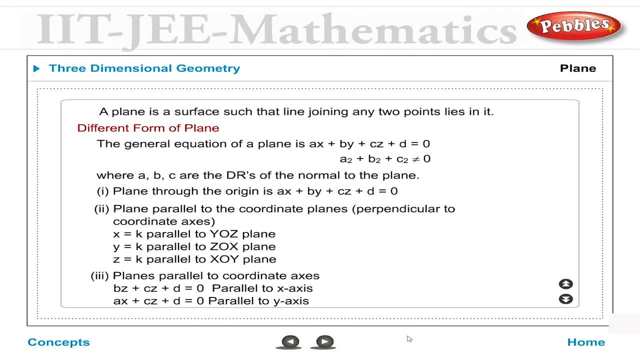 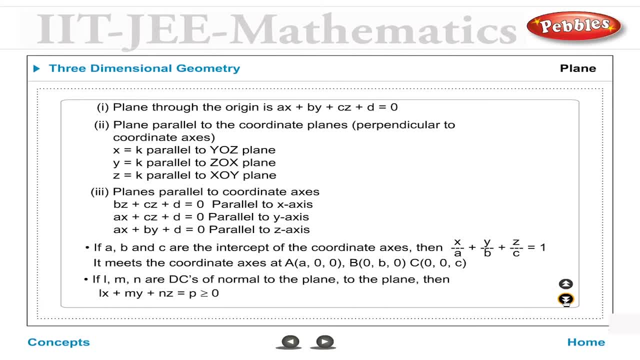 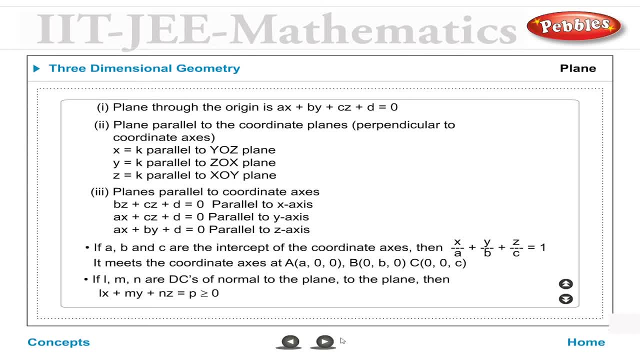 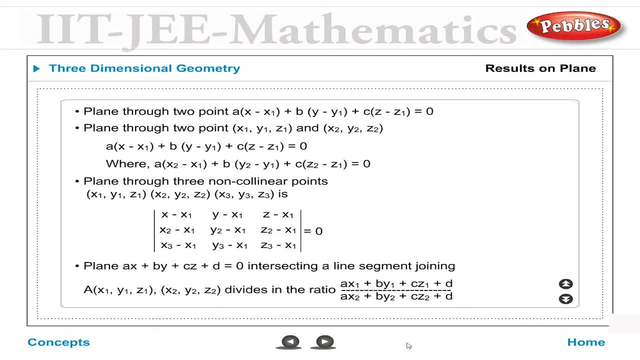 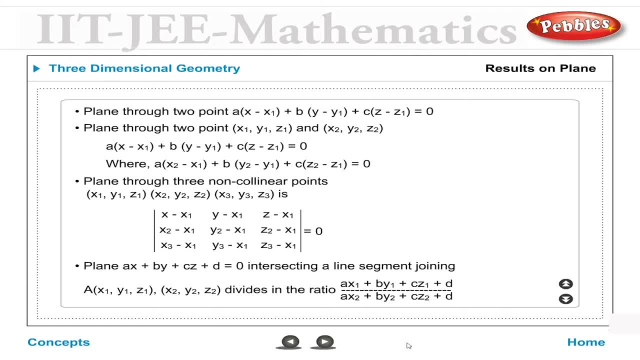 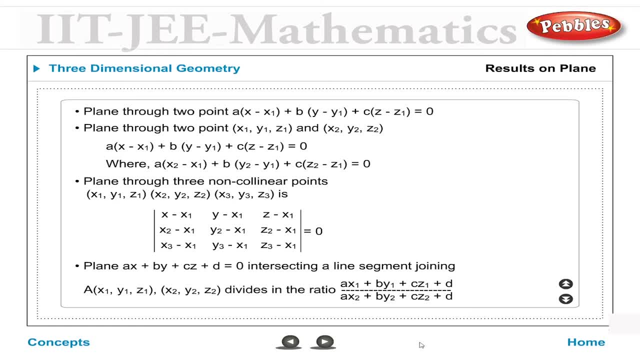 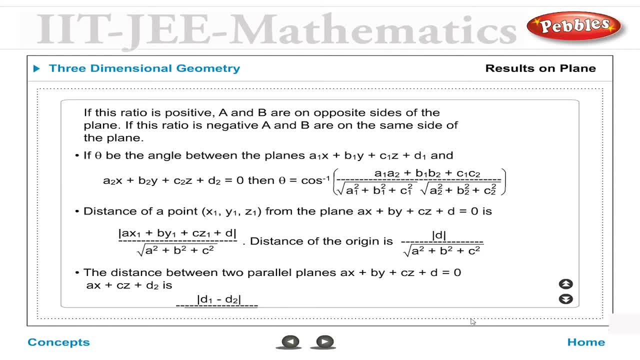 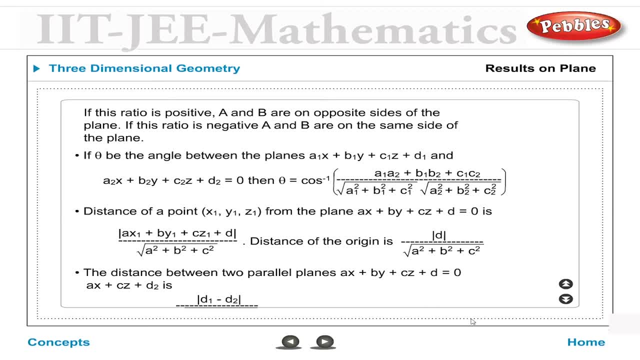 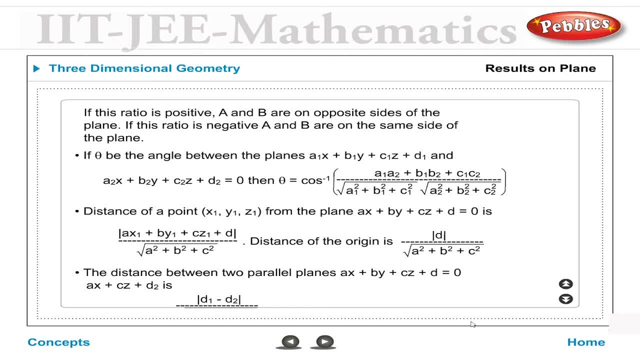 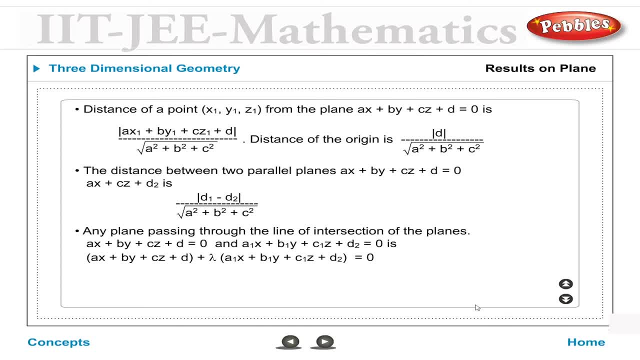 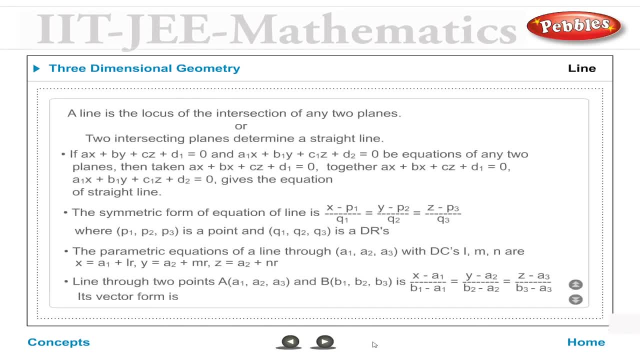 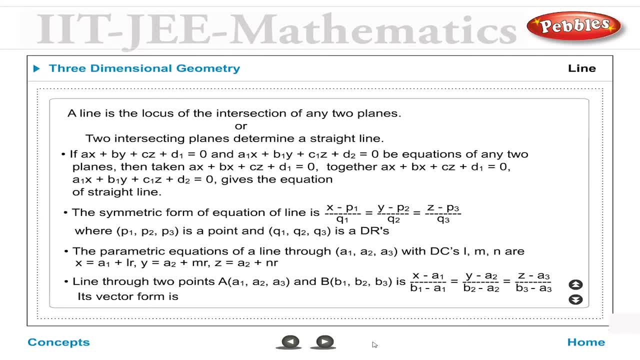 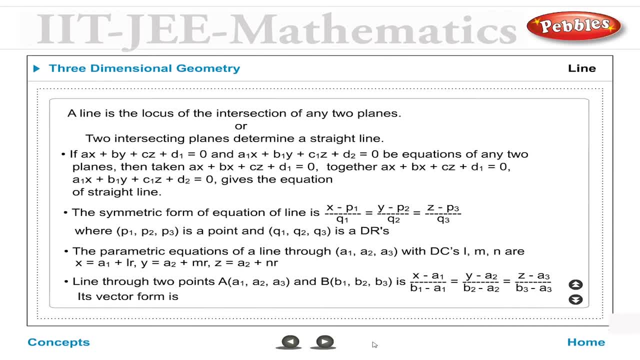 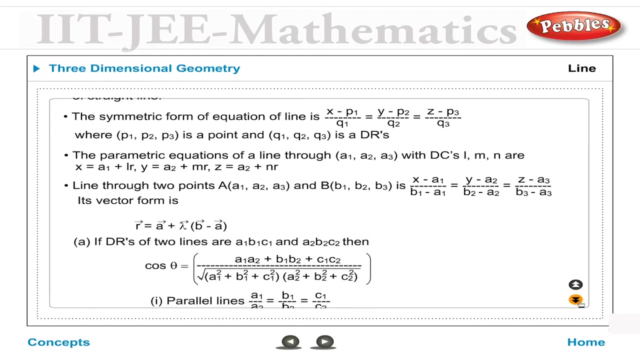 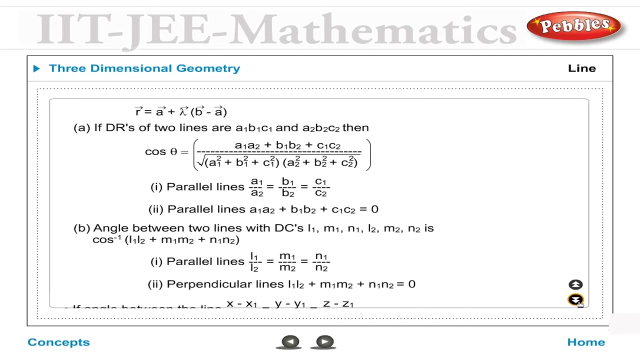 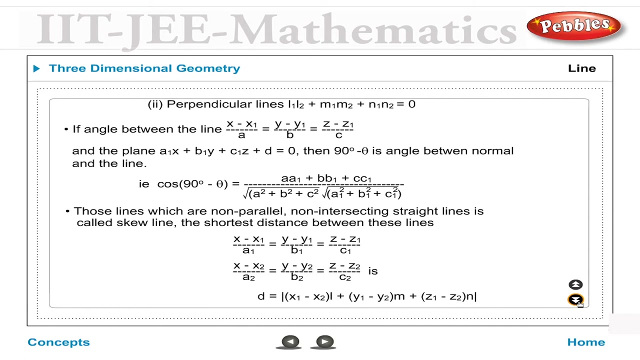 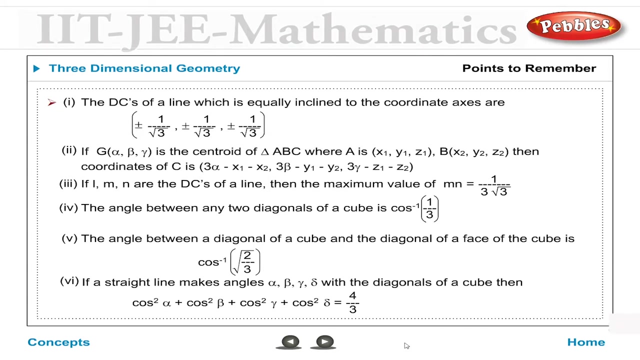 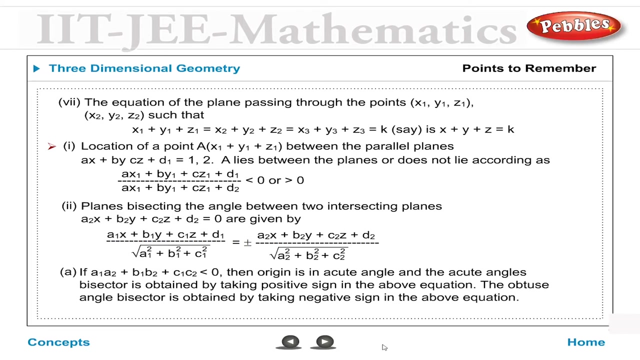 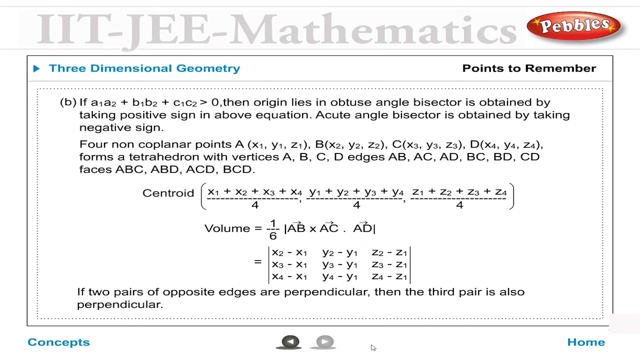